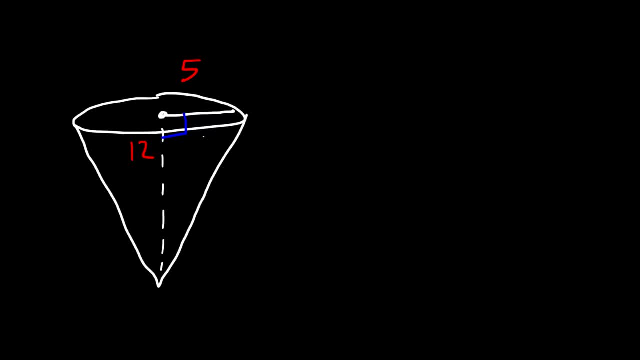 use that to calculate the surface area, The lateral area. it's 1 half PL. We have R and we have H. This is the slant height. L and P represents the perimeter of the base, which is a circle. So the perimeter of the circle which is this conference. 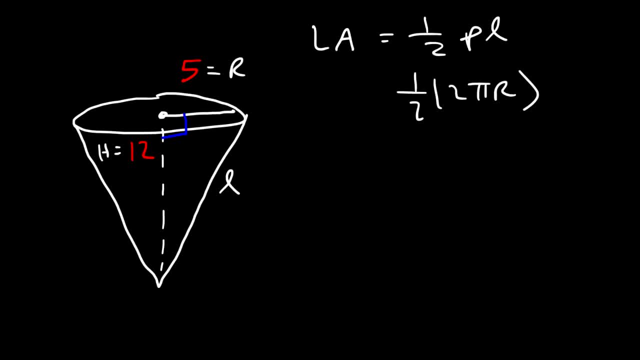 that's 2 pi R. So therefore the lateral area is- I wrote the equal sign twice. it's pi R L, and so that's how you can find it. So we need to calculate L first and notice that we have a right triangle. So L squared is equal to R squared plus H squared, So in 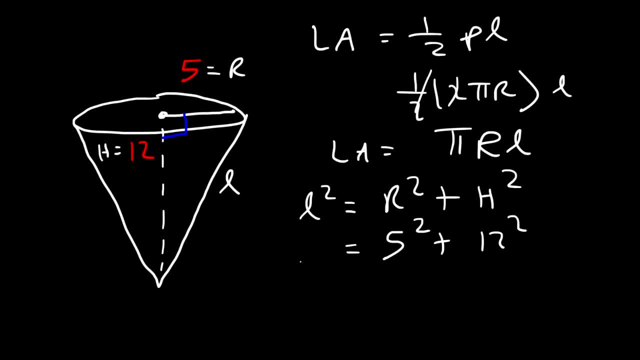 this example: R is 5, H is 12.. 5 squared is 25, 12 times 12 is 144, and 25 plus 144 that's 169.. So now what we need to do at this point is take the. 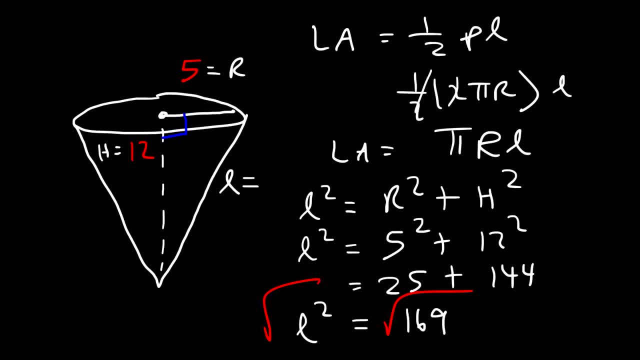 square root of both sides. So the square root of 169 is 13, and so that's the slant height. So the lateral area is going to be pi times R times L. So 5 times 13 is 65.. So it's 65 pi squared L times L. 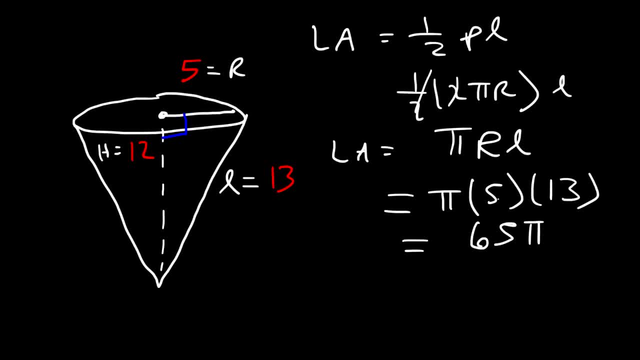 So 5 times 13 is 65, so it's 65 pi squared. So 5 times 13 is 65.. So with 65 pi squared you can calculate the lateral area units. So if this is in inches the surface area is going to be square. 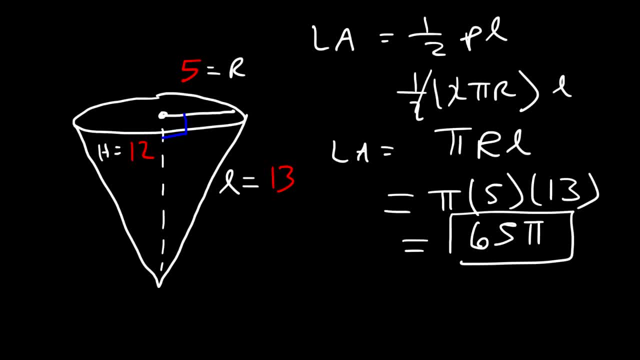 inches. Now let's focus on calculating the total surface area. So that's equal to the area of the base plus the lateral area. The area of the base is pi r square, The lateral area is pi r L. So this is the formula to calculate the total. 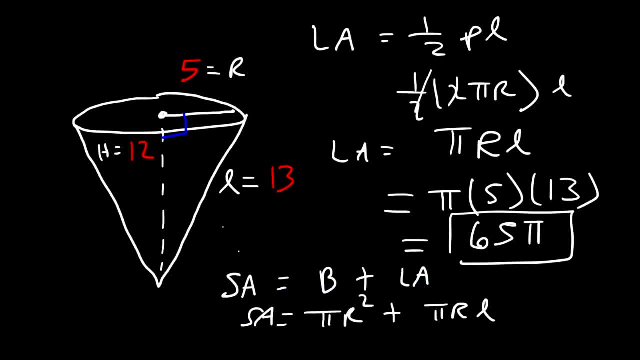 surface area of a cone. So pi r square, that's going to be pi times 5 squared, And we know pi r L is 65 pi. based on this answer, 5 squared is 25 and 25 plus 65 is 90.. So the total surface area is 90 pi in this example.